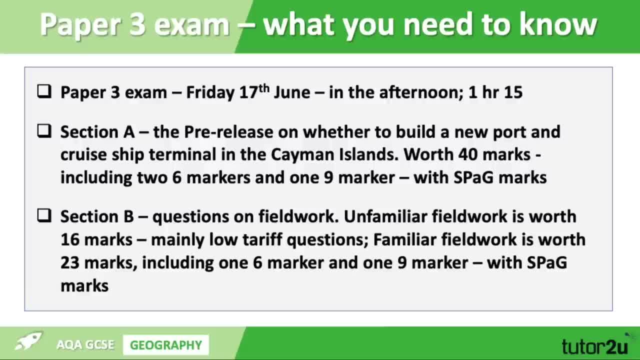 process and think about the different aspects that you could be tested on. The fieldwork section is worth 39 marks. Question 4 is about unfamiliar fieldwork and presents a series of data response questions varying between 1 and 4 marks. These are based on different fieldwork scenarios You might 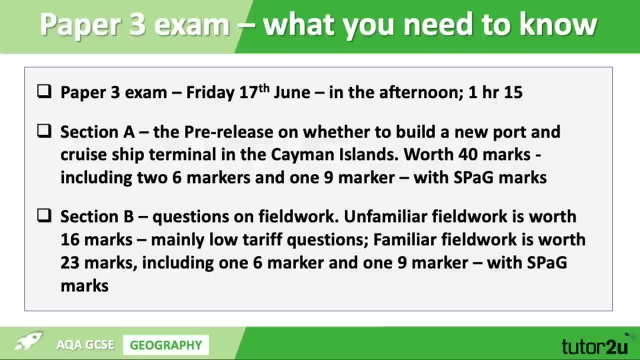 be asked to complete a table of data or a graph to evaluate the strengths and weaknesses of a data collection model or sampling frame, or to suggest ways in which to improve a piece of fieldwork. Question 4 is worth 16 marks in total. 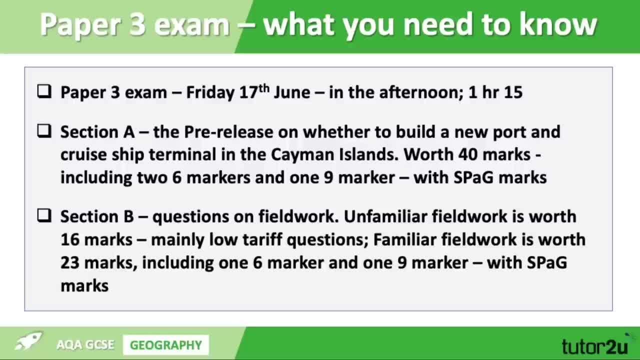 Question 5 is all about your own experiences of fieldwork. During the GCSE course, you will have completed two contrasting fieldwork enquiries: a physical fieldwork enquiry and a human fieldwork enquiryenn private funders. Read the instructions carefully, as some of the existing questions 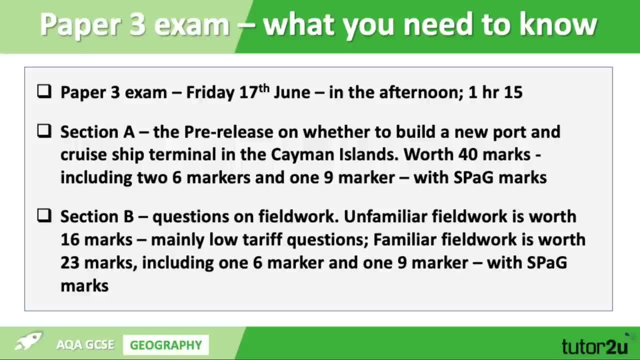 specify that some questions will become ставable back to end of your fieldwork studies, Those which of your fieldwork enquiries they want you to talk about. The questions here are all about evaluating your own fieldwork enquiry. For example, you might be asked to assess how suitable your 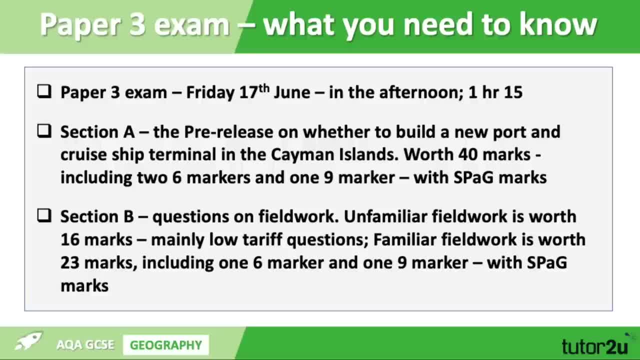 study sites were what the risks were when you were collecting data or how useful your data collection was at drawing conclusions. This section is worth 23 marks, which includes one six marker and one nine marker, with three SPAG marks available. We are going to start off with a game of altered vowels, So each of the stages of fieldwork. 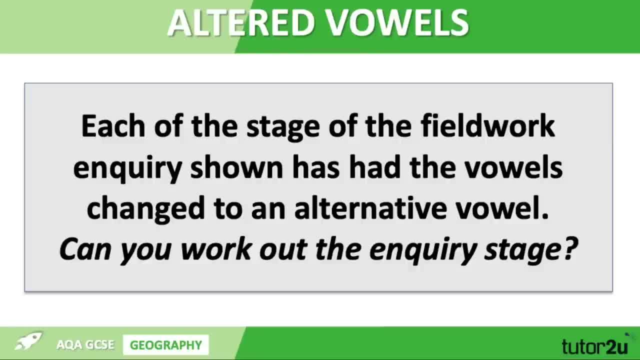 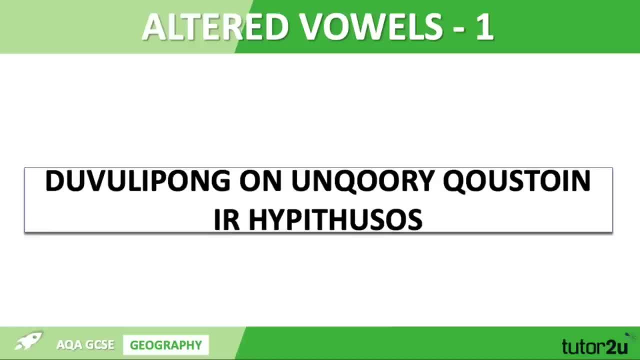 enquiry shown has had the vowels changed. an alternative: Can you work out the enquiry stage? Here's our first one, So we'll just leave it up for a moment, see if you can work it out. Okay, remember, it's not an anagram, it is just a number. 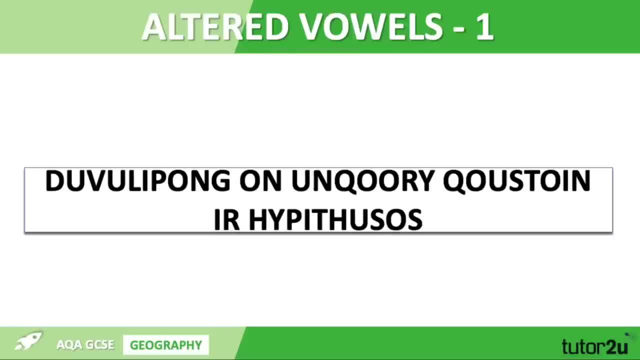 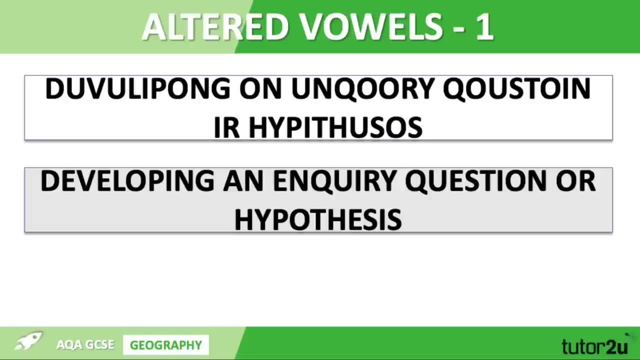 It's just the vowels that have been changed, Right? let's see if you were correct. It is developing an enquiry question or hypothesis. So in a moment I'm going to talk about what all these different stages are in a bit more detail. Number two: 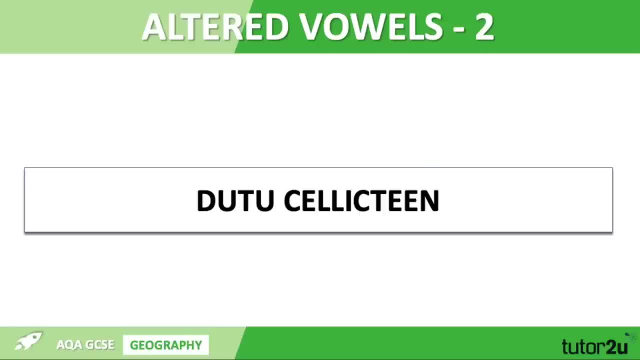 Okay, this one is a little bit easier, hopefully. Okay, let's have a look. It is data collection. so well done if you got that correct. Number three: Okay, let's check this one. It is data presentation. Number four: Okay, let's have a look. It is data analysis. And number five is: 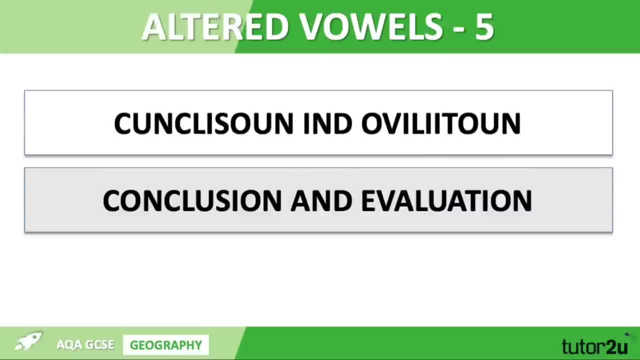 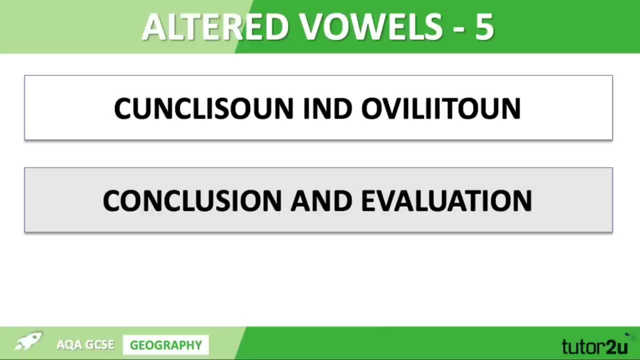 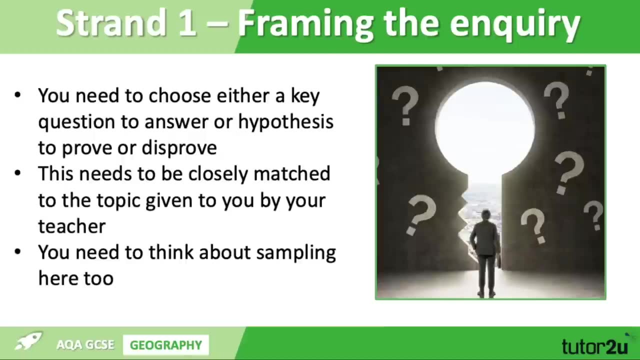 Okay, let's have a look at this one. It is conclusion and evaluation. Throughout this video, I'm going to talk about those different stages and the different things that might be important to consider with each of those stages. So we're going to start off by looking at strand one. Okay, now you need to be familiar with all. 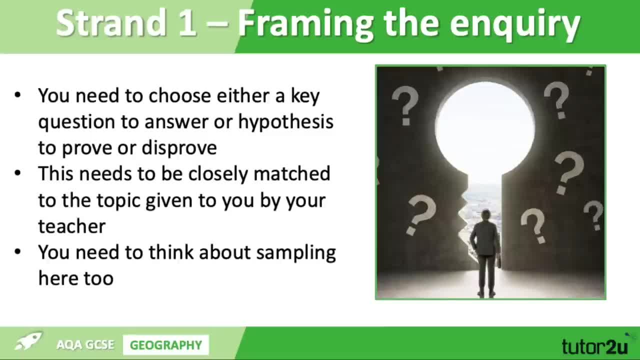 of these different strands. Strand one is framing the enquiry, which basically means selecting a suitable question for geographical enquiry. You need to choose: either a key question to answer or a hypothesis to prove or to solve. So we're going to start off by looking at strand one. 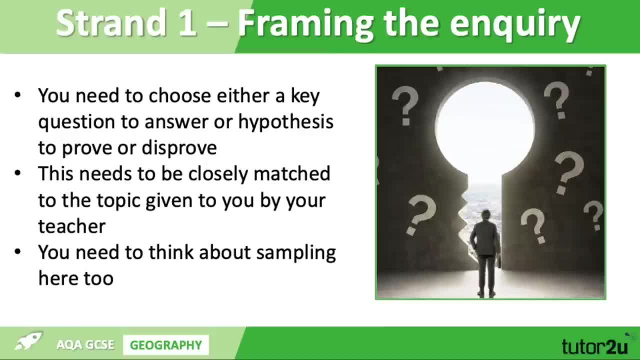 Okay, now you need to be familiar with all of these different strands. Strand one is framing the enquiry, which basically means selecting a suitable question for geographical enquiry. You need to choose either a key question to answer or a hypothesis to prove or to solve. This needs to be closely matched to the topic given to you by your teacher. 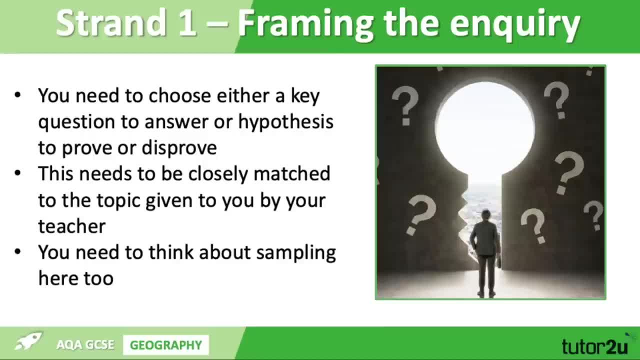 and you also need to think about sampling too. In the exam, you may be asked about factors to consider when selecting your enquiry question: The theory or concepts underpinning the enquiry, appropriate sources, primary and secondary data, and how any issues that arise at this stage could. 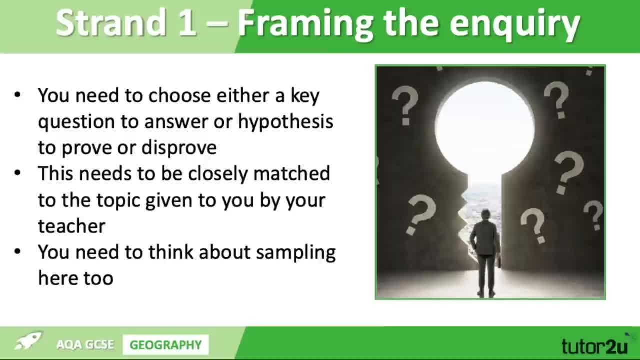 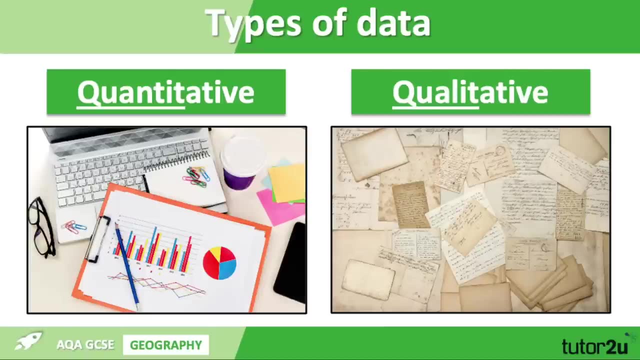 be reduced. An example exam question here is: justify the choice of your human or physical enquiry question. When planning a fieldwork enquiry, you need to think about what types of data will be most useful to answer the enquiry question. Data can be divided into two groups: quantitative and qualitative. 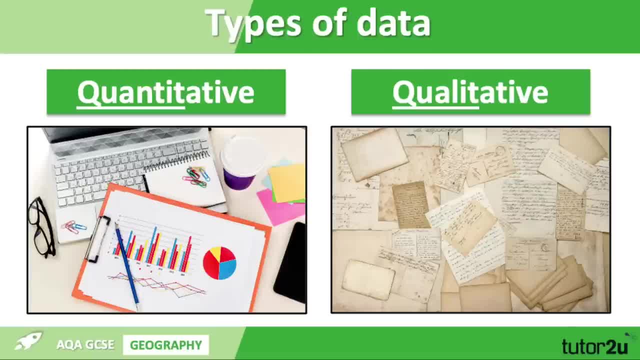 Quantitative data is statistical data that is numerical and can be presented in tables and graphs. Because it's in numerical form, it's measurable and easy to put in categories or in rank order. A good way of remembering what quantitative data is is by using the first. 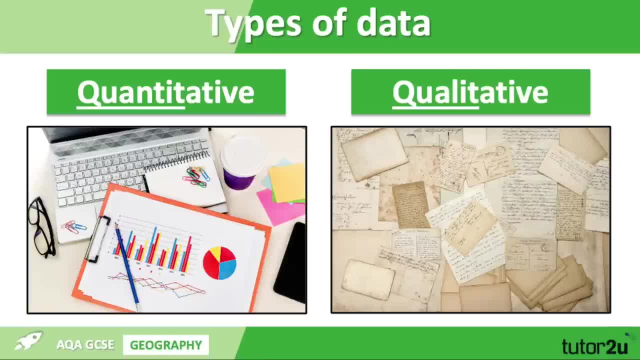 seven letters of the word. Quantitative data is high in quantity, ie there's a lot of it. Qualitative data, on the other hand, is data that is in words and is detailed, and it helps to provide context. Qualitative data gathers information that is not in numerical form. Instead, it's normally in. 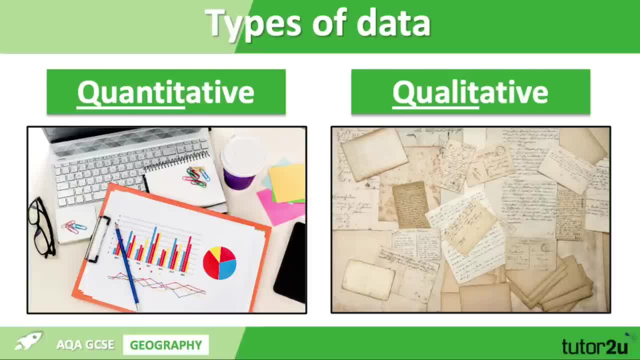 words or sentences, such as old diaries, newspaper reports and other types of data. The qualitative data is usually very detailed and therefore quite time-consuming to collect. A good way of remembering what qualitative data is is by using the first six letters of the word. 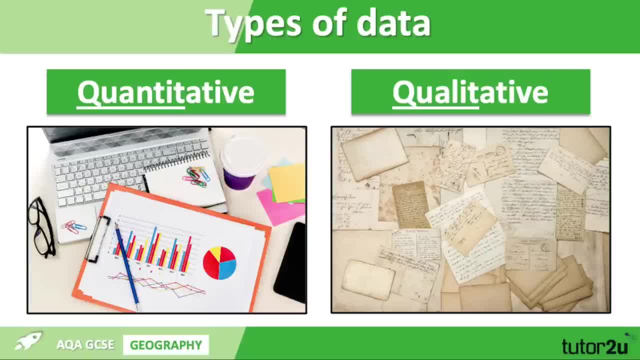 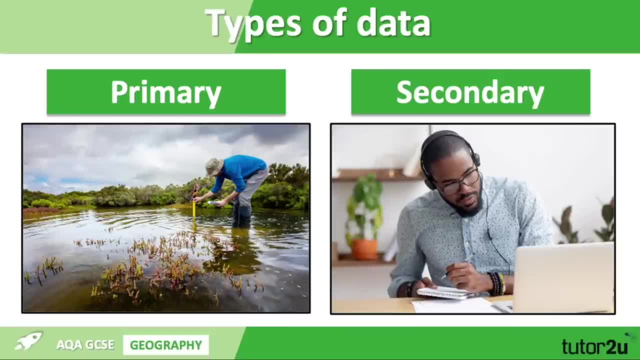 Qualitative data is quality data. Fieldwork enquiries will usually involve both primary and secondary data. Primary data is research information that you have collected out of the data you have collected. So if you have a data that is not in the field yourself, There are lots of different data collection methods available to us. 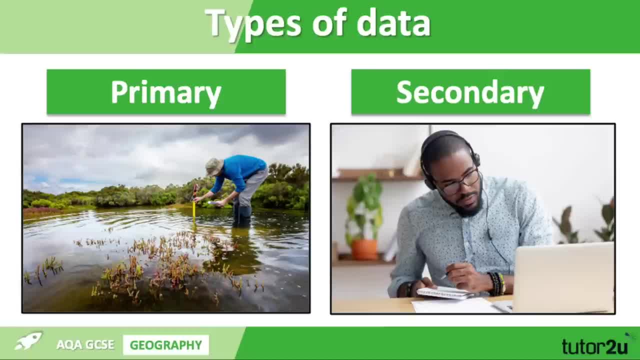 which we're going to have a look at in a minute. Collecting primary data is time-consuming. however, you do collect exactly what you need and, in theory, this should be reliable. Secondary data is information that has been collected by someone else for another purpose. It is often used by 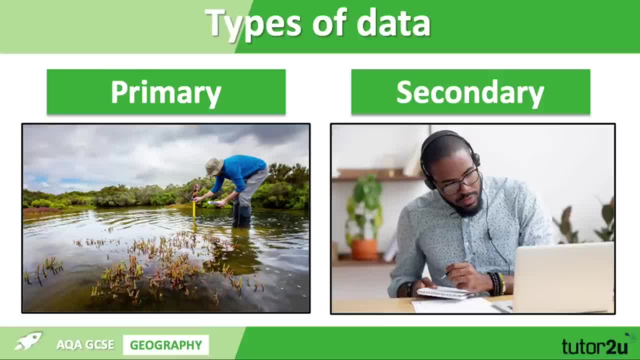 geographers to back up their own fieldwork data. There are a wide range of sources of secondary data. Some of these are quantitative, such as official statistics like the UK census, whereas some of them will be qualitative, such as old diaries, books and 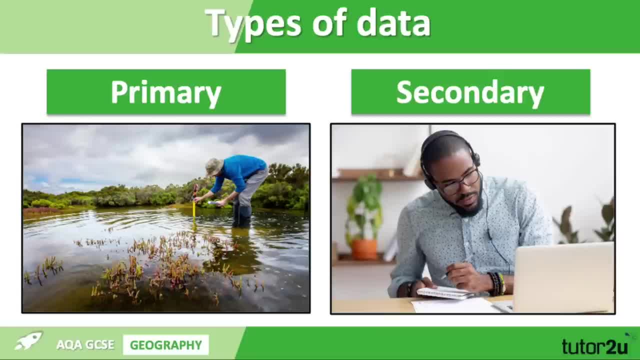 newspapers. The biggest advantage of this data is that it already exists and it is easily available. However, as it has been collected by someone else, there are issues to consider. The data may be out of date, it could be biased or it could simply be overwhelming, as there's so much of it. 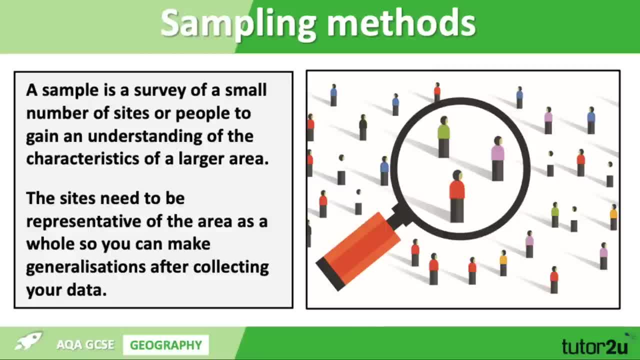 Once you've decided what sort of data you want to find, you have to decide where you're going to collect your data. A sample is used in fieldwork, as it is often hard or too time-consuming to survey a whole area or to collect large amounts of data. A sample is a survey of a small number of sites. 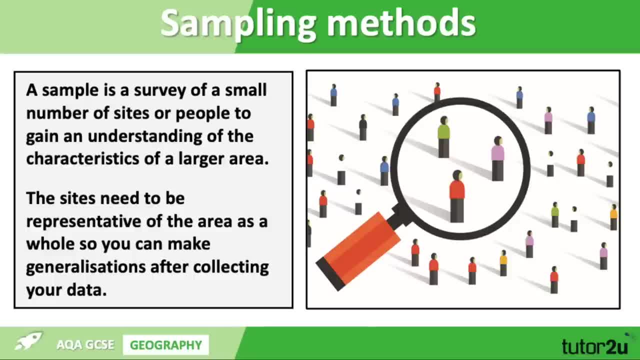 or people. to gain an understanding of the characteristics of a larger area, The sites need to be representative of the area as a whole so you can make generalisations after collecting your data. Let's have a look at some of the sampling techniques you might get asked about. 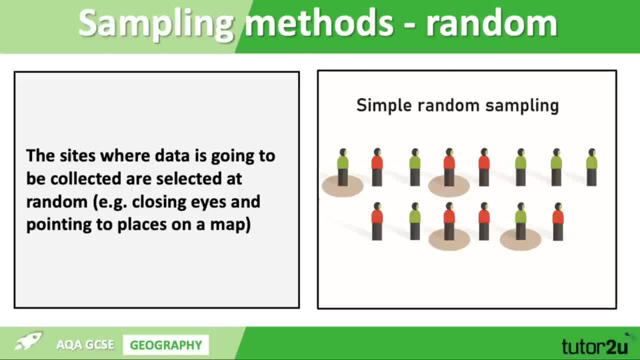 Our first one is random sampling. This is where the sites where data are going to be collected are selected at random, ie by closing eyes and pointing to places on a map or drawing names out of a hat. There are lots of advantages to random sampling. It can be used with large samples or a 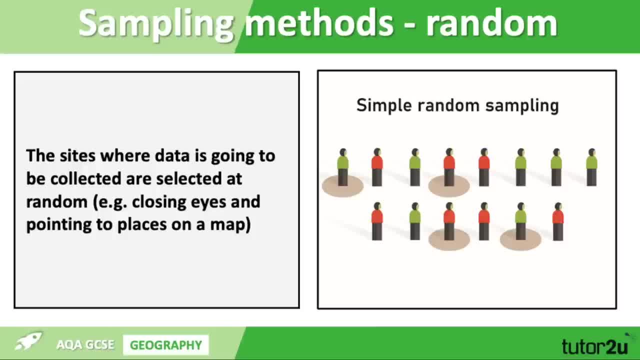 large sample area. it avoids any bias as it is totally random and it is easy to carry out the same fieldwork again. However, data will not be evenly distributed and there could be gaps in your data or areas missed, particularly if the study area is large and some of the sites 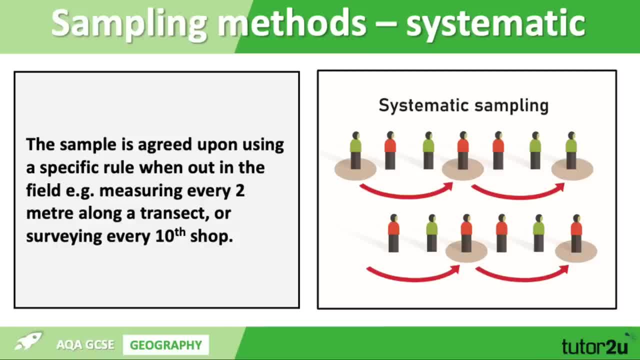 that you've picked may be difficult to access. Our second sampling method is systematic sampling. This is where the sample is agreed upon using a specific rule when out in the field, For example, measuring every two metres along a transect or surveying every tenth shop There. 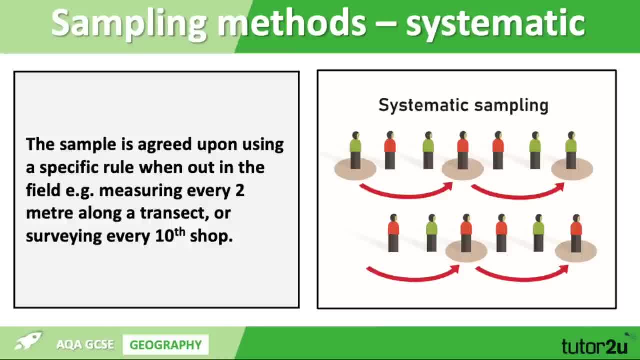 are lots of advantages to systematic sampling. Data is evenly distributed across an area and it is easy to carry out the same sampling. The second method is systematic sampling- For example, every tenth house- and it is more straightforward than other sampling types. It ensures a good coverage of the study area also. However, the selected rule might not work. 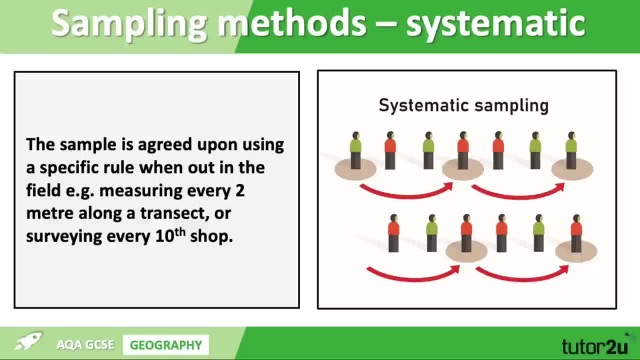 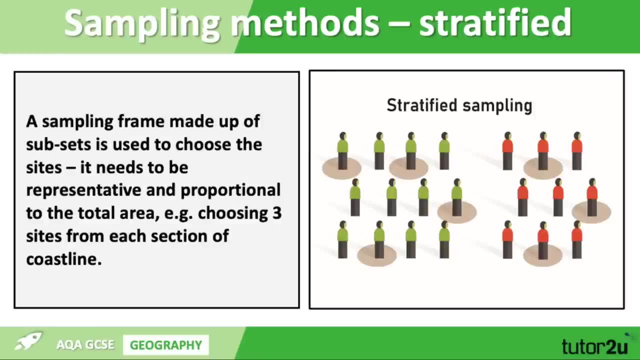 out in the field. It might be biased in the results, as the different areas or pieces of data do not have an equal chance of being selected and it may not be representative of the area as a whole. Our last sampling technique is stratified sampling. This is where a sampling frame made up of three 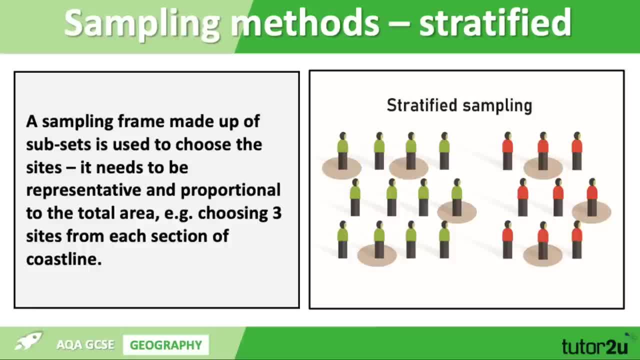 subsets is used to choose the sites. It needs to be representative and proportional to the total area, eg choosing three sites from each section of a coastline. There are lots of advantages to stratified sampling. It gets a good coverage of data and the areas, so results are more. 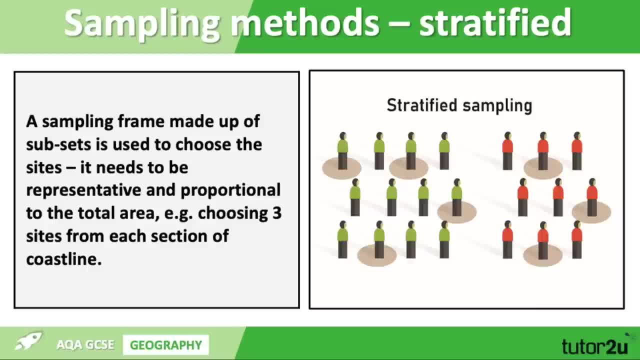 representative. It can be used with other sampling techniques and it is easy to compare the subsets. However, you do have to research the area before data collection in order to choose the sampling subsets. The proportion of the data collected is not always the same. The proportion of the data. 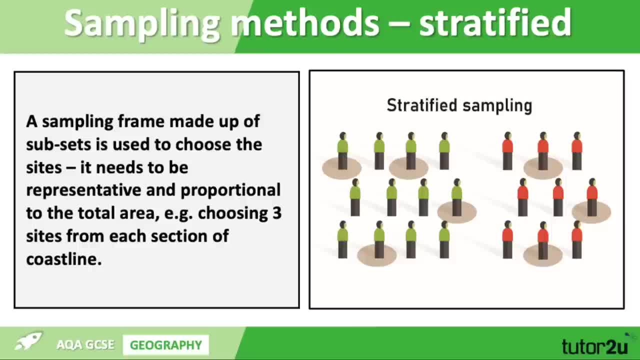 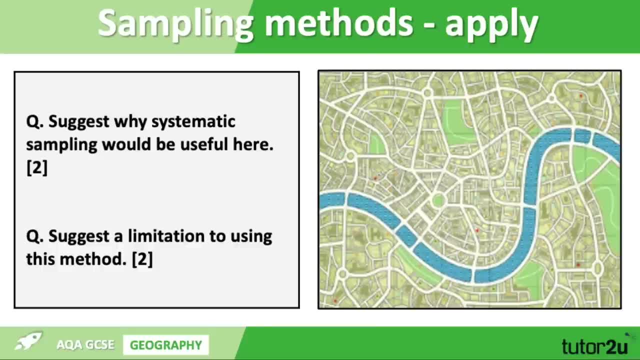 collected is not always the same. The proportion of the data collected is not always the same. The proportion of subsets also needs to be accurate and bias can be introduced into the sample. In terms of sampling methods, you may be given a map extract and ask to suggest a sampling method. 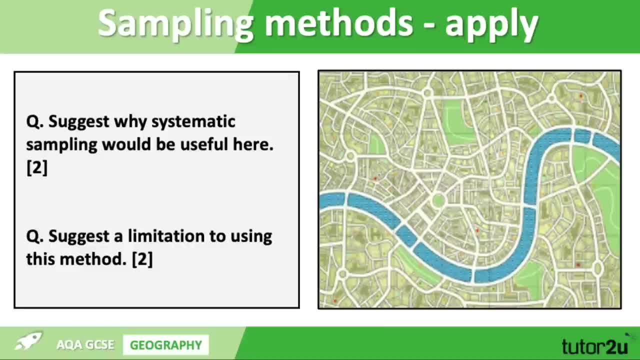 for measuring something in particular. We've used the example of measuring traffic on the screen, along with two examples of low tariff questions. So we've got suggest why systematic sampling would be useful here and suggest a limitation to using this method For the top question: systematic- 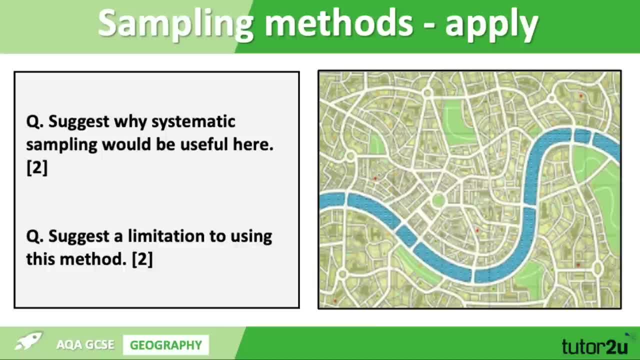 sampling would be useful here and suggest a limitation to using this method For the top. sampling would offer a good coverage of this urban area and could be organised in the classroom beforehand. For the second question, physical features such as the river may get in the way. 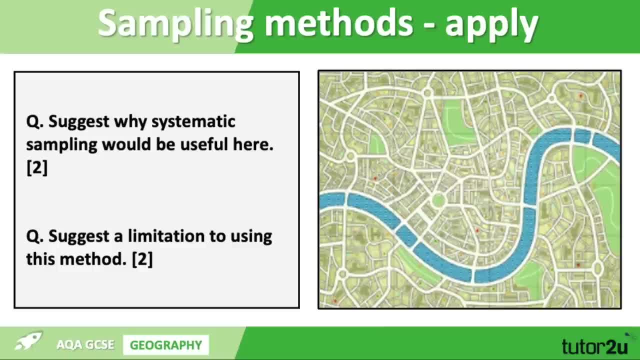 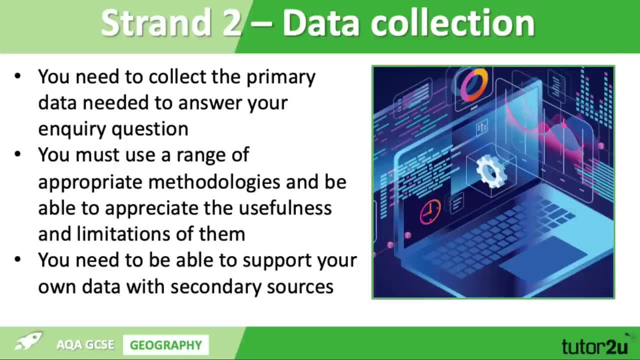 which would affect the representativeness Right. let's move on to strand two. This is data collection, which is all about selecting, measuring and recording data appropriate to the chosen inquiry. You need to collect the primary data needed to answer your inquiry question. You must 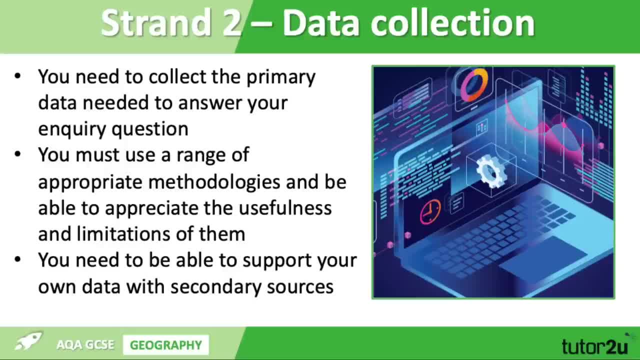 use a range of appropriate methodologies and be able to appreciate the usefulness and limitations of them, and you need to be able to support your own data with secondary sources. In the exam, you may be asked questions involving the difference between primary and secondary data, how you 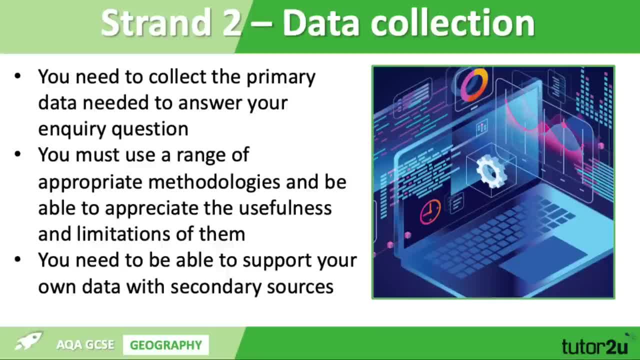 identified and selected appropriate physical and human data and how you measured and recorded your data using different sampling methods. You may also be asked to describe and justify your data collection methods. An example question here is: justify one data collection method used for your human or physical fieldwork for four marks. 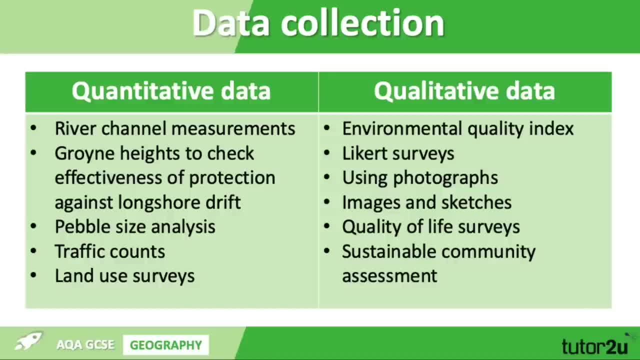 Let's quickly remind ourselves that some of the data collection methods that are available to geographers and therefore might make an appearance in paper three. So, in terms of quantitative data, we've got river channel measurements, groin heights to check effectiveness of protection against longshore drift, pebble size analysis, traffic counts and land use surveys- Quality data. 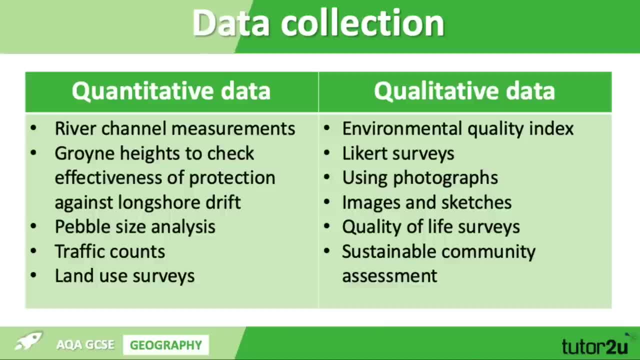 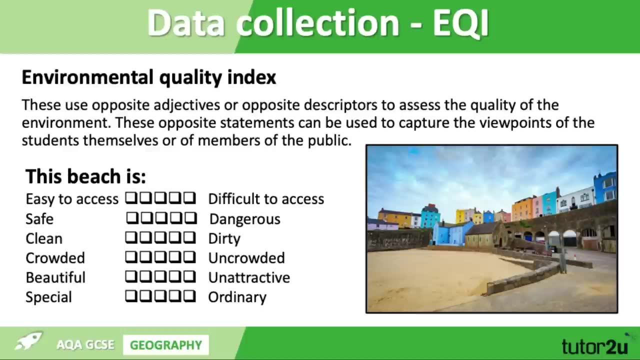 could include environmental quality index, lick hurt surveys using photographs, image and sketches, quality of life surveys and sustainable community assessments. So let's have a look at a few of these in a bit more detail. This one is an environmental quality index. They use opposite adjectives or 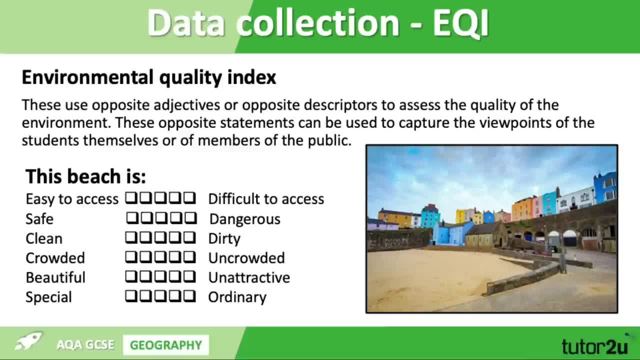 opposite descriptors. Students can be involved in selecting or writing appropriate opposite statements, and these statements can be used to calculate the quality of the data collected. So let's have a look at a few of these in a bit more detail. This one is an environmental quality. 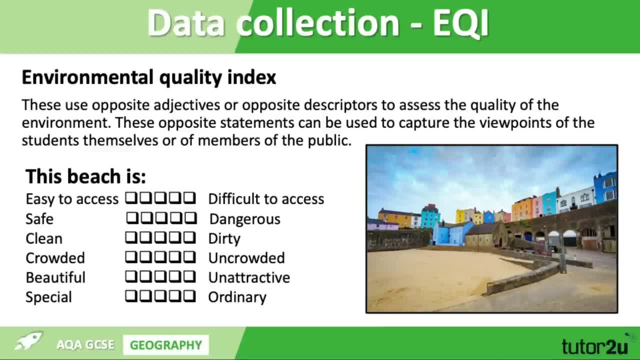 index. Students can be involved in selecting or writing appropriate opposite adjectives or different opinions In an exam. you might be asked to complete two more lines in an environmental quality index, ie give two more opposite statements, or you might be asked to think about the limitations of this type of survey. In this case, the biggest limitation is that it is so. 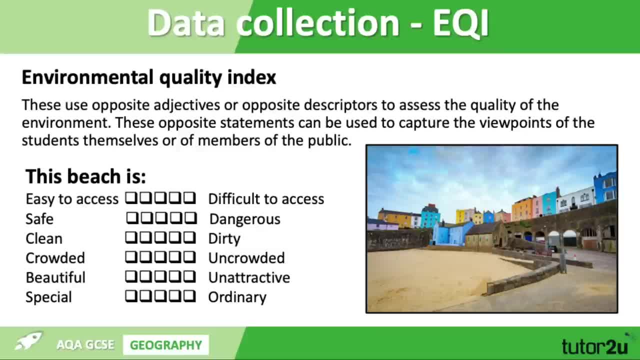 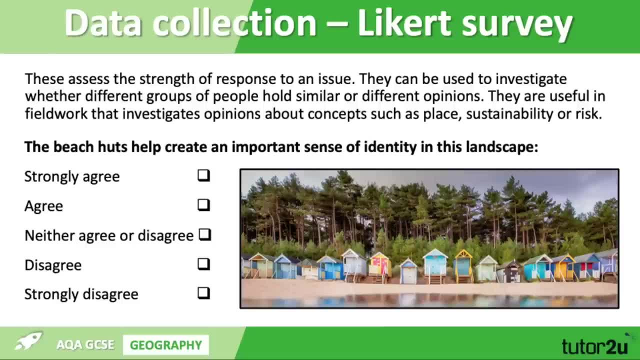 subjective and open to interpretation, meaning that the results are less accurate. So let's have a look at the results. Another data collection technique that is based on opinions is a lick hurt survey. These assess the strength of a response to an issue. They can be used to investigate whether different groups of 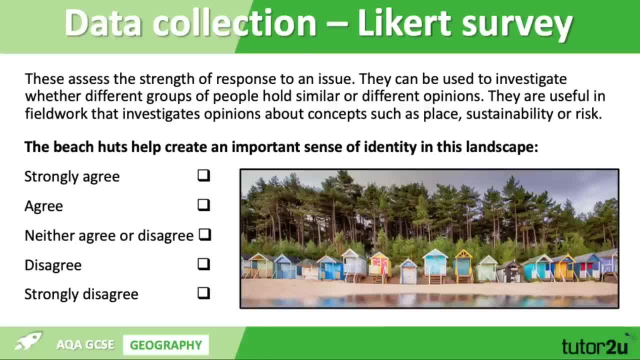 people hold similar or different opinions, and they're useful in field work that investigates opinions about concepts such as place, sustainability or risk. Again, for this type of data collection method, you may be asked to suggest strengths or weaknesses. So they do collect a lot of data and they're used to investigating whether different groups of people hold similar or different. 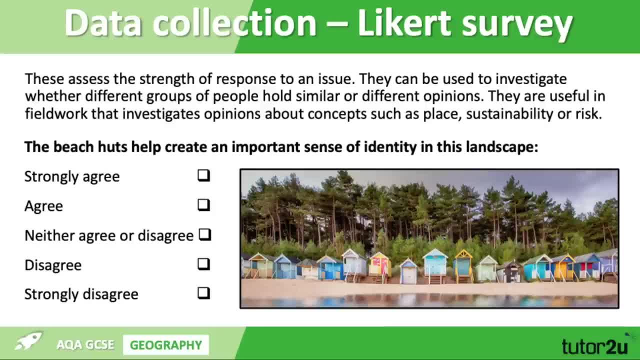 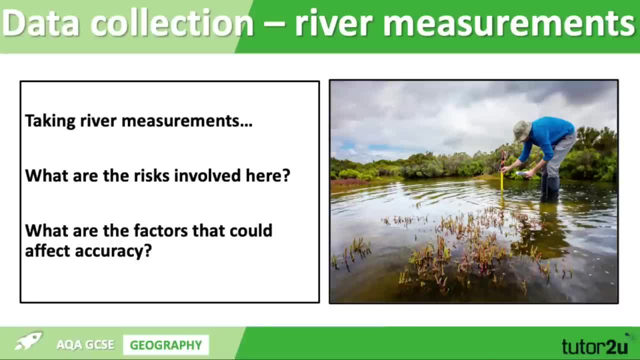 opinions quickly. However, the closed nature of the survey means you don't know why someone has that opinion. In the exam you may be given a physical geography scenario, such as measuring the water depth at intervals across a river. There are a couple of things that could come up regarding. 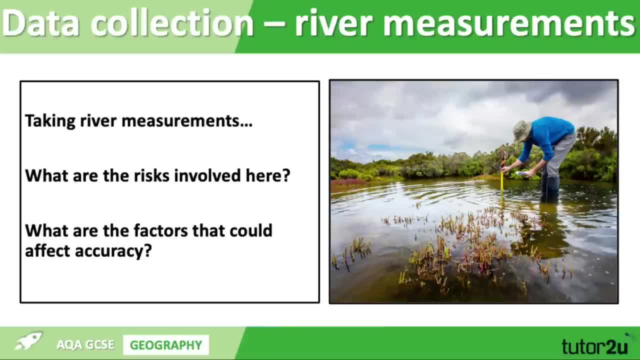 this method of collecting data. Firstly, there may be a question about the risk assessment aspect of this field work, Thinking about risk here, such as slipping on wet rocks and falling into the river. The question could also be about the accuracy of collecting data. This is a big issue with physical 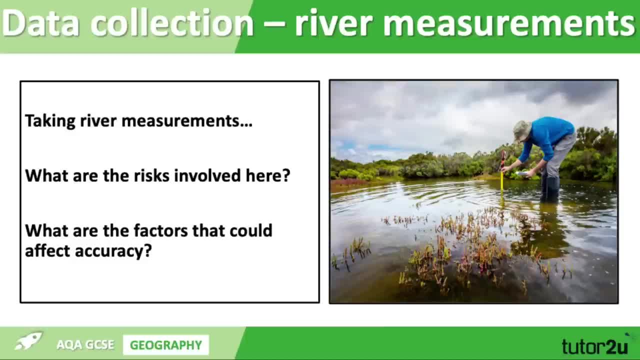 geography data. You need to make sure the tape measure is pulled tight across the river to make your depth measurements as accurate as possible. However, there could be big rocks on the riverbed, meaning you are measuring the distance from the water surface to them and not the actual riverbed. 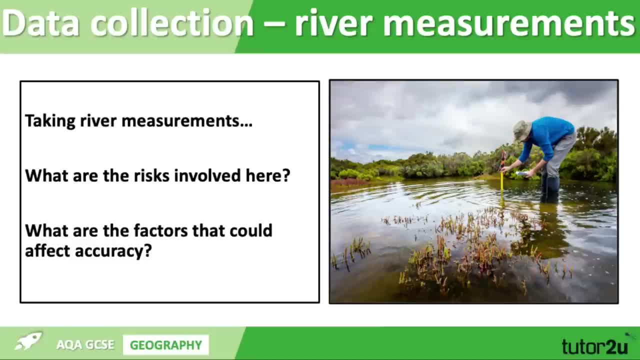 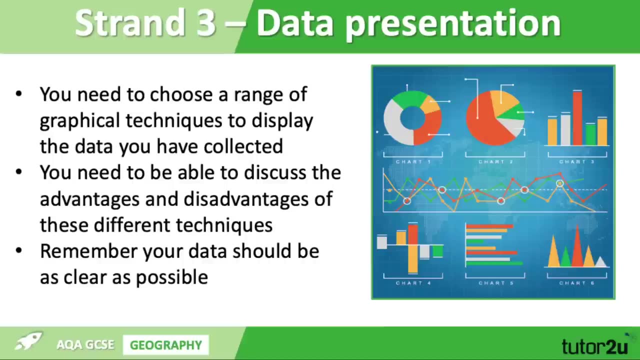 There are also problems with coastal data collection. for example, when measuring groin heights to assess the effectiveness of protection against longshore drift, Missing slats could make the results inaccurate. Our next strand is strand three, which is data presentation. This is selecting appropriate ways of processing and presenting your field work data You need to. 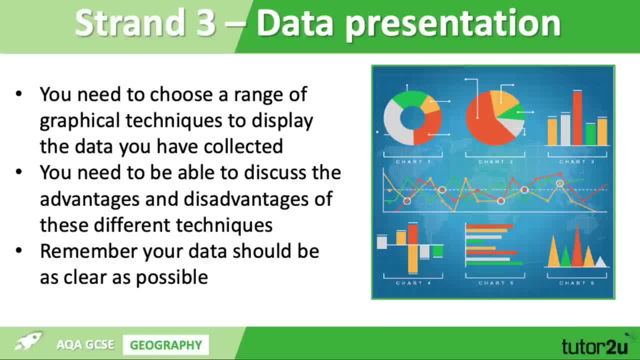 choose a range of graphical techniques to display the data that you have collected. You need to be able to discuss the advantages and disadvantages of these different techniques and remember your data should be as clear as possible. In the exam, you will be expected to appreciate that a range. 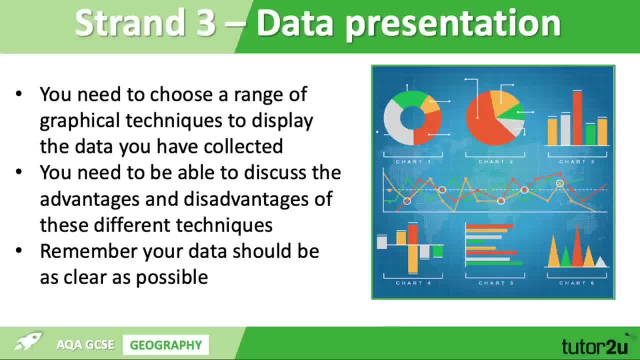 of visual, graphical and cartographic or mapping methods are available and you may be asked to describe and explain your selection. You might be asked to talk about accurate use of presentation methods and, finally, you could be asked how you adapted presentation methods to suit your inquiry. 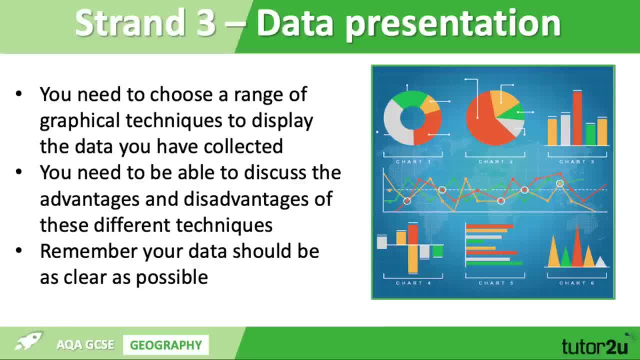 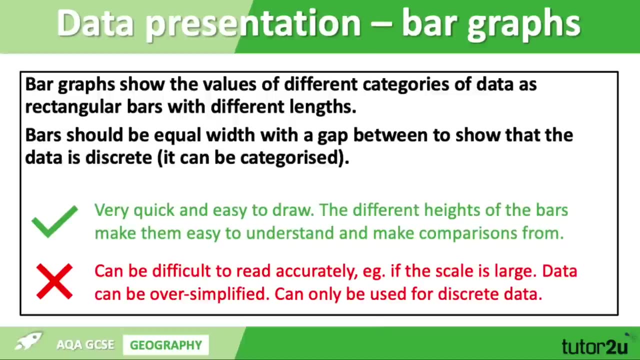 An example question here could be: explain how one data interpretation technique, using your human geography inquiry, helped you interpret your data for six marks. It is likely that you will either be given some data and asked to suggest the best ways to present it and why, or you may be shown a graph and asked to explain why that's the most appropriate way to 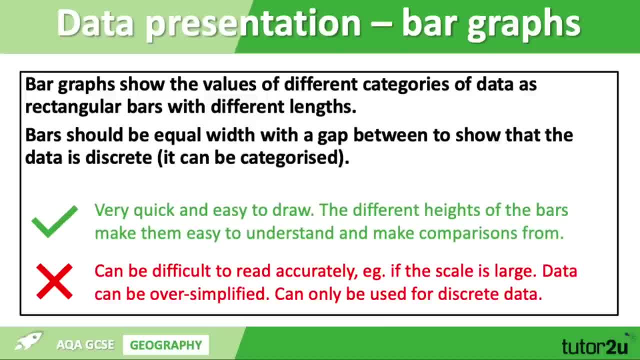 present the data. So we're going to remind you of the different ways that you can present data, and their strengths and weaknesses. I'm going to start off with bar graphs. Bar graphs show the value of different categories of data as rectangular bars with different lengths. Bars should be equal. 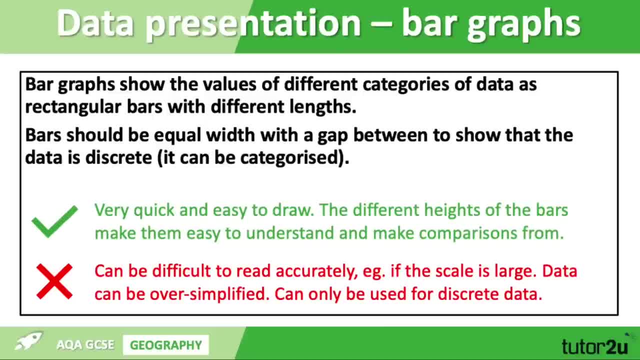 width with a gap between, to show the data is discrete. Bar graphs show the value of different categories of data as discrete and that it can be categorized. So an advantage is it's very quick and easy to draw and the different heights of bars make them easy to understand and make comparisons. 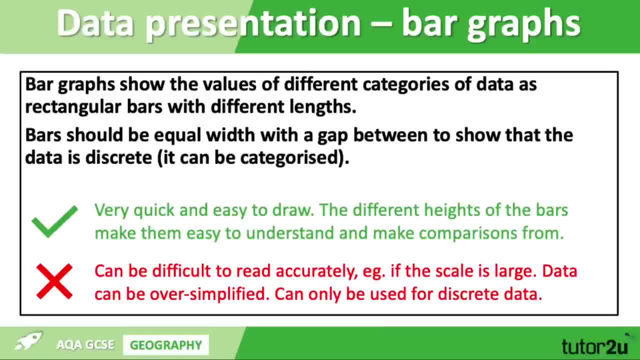 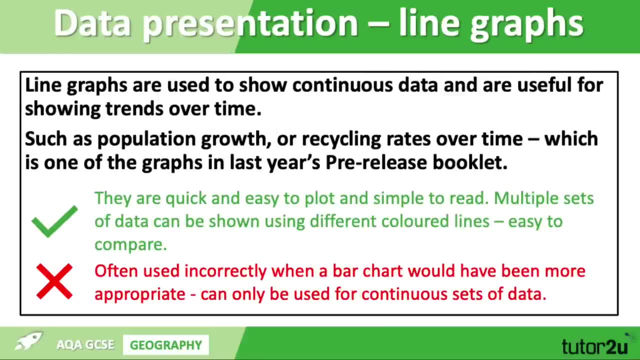 from. However, it can be difficult to read accurately, particularly if the scale is large. Data can be oversimplified and it can only be used for discrete data, so not data that shows change over time. So, speaking of change over time, let's move on to line graphs. Line graphs are: 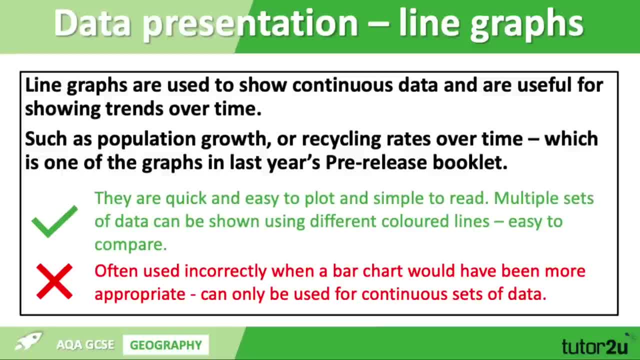 used to show continuous data, So line graphs are used to show continuous data. So line graphs are used to show continuous data and are useful for showing trends over time. So, for example, an increase in population or recycling rates over time. Now the recycling rates over time. 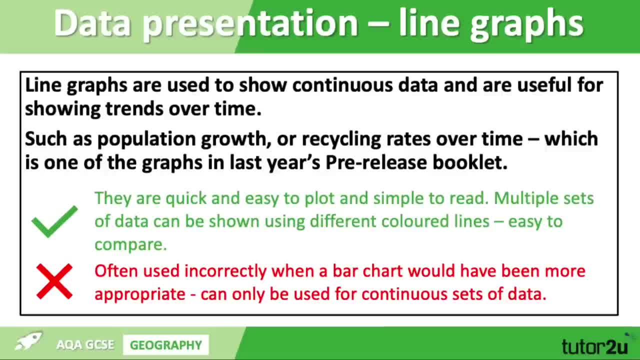 interestingly was one of the graphs in last year's pre-release booklet that you might have seen if you've done that as part of a mock. They are quick and easy to plot and they are simple to read. Multiple sets of data can be shown using different colored lines, so they are easy to. 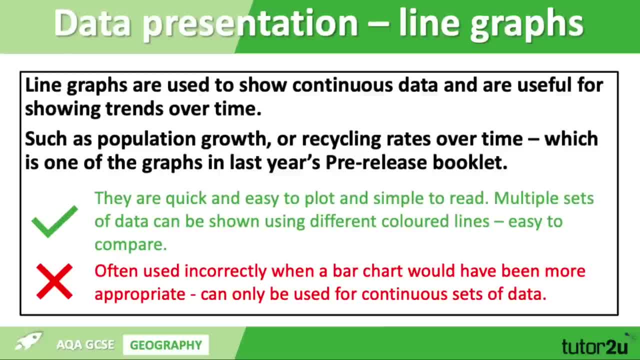 compare. However, they are often used incorrectly when a bar chart would have been more appropriate. and they are often used incorrectly when a bar chart would have been more appropriate, So they can only be used for continuous sets of data. Let's move on to pie charts, So these crop up in. 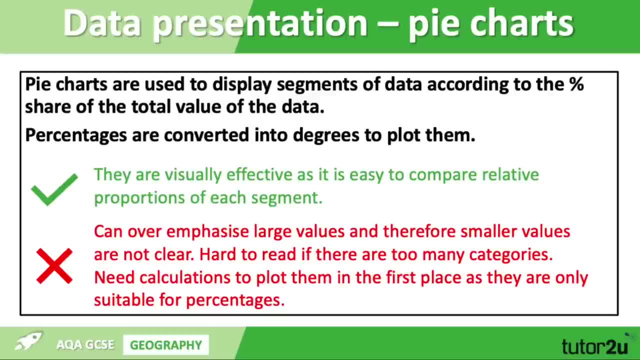 the exams most years. Pie charts are used to display segments of data according to the percentage share of the total value of that data And the percentages are converted into degrees to plot them onto your pie chart, onto your circle. So they are visually effective and it's quite easy. 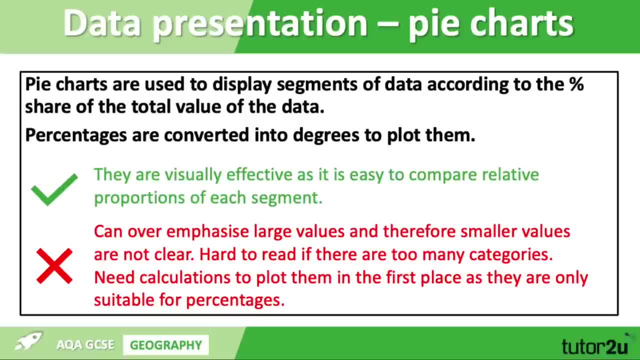 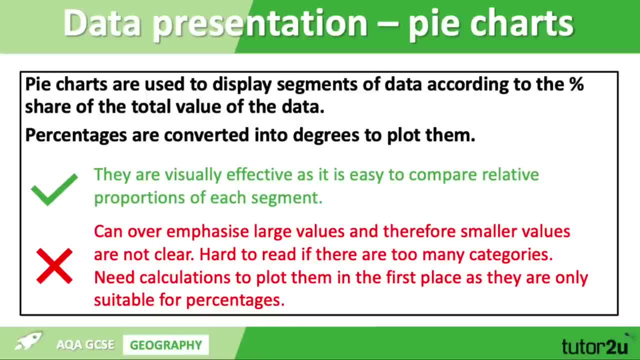 and therefore smaller values are not clear And they're really hard to read. if there are too many categories, You obviously need calculations to plot them in the first place, so they're only suitable for data that is in percentages. So another data presentation technique that you 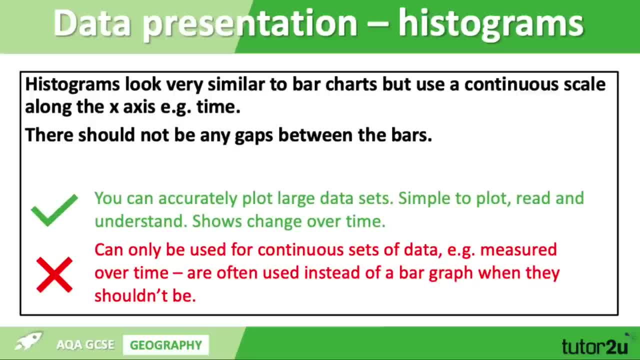 should be familiar with is histograms. Histograms are very similar to bar graphs, but they use a continuous scale along the axis- sorry, along the x-axis- for example, time- And there shouldn't be gaps between the bars, because if you have a lack of gaps, it's highlighting to you that data is. 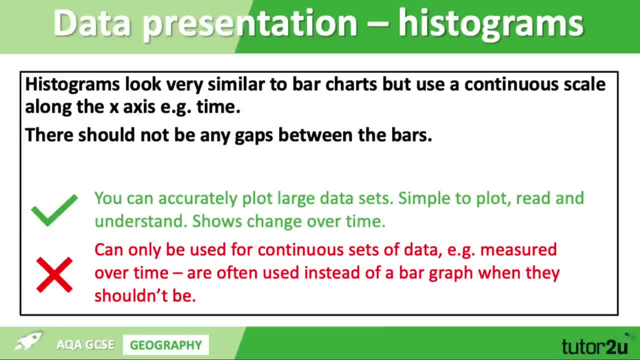 continuous. If you draw gaps between then, that obviously is discrete data. Now they're useful because you can accurately plot large data sets. They are simple to plot, read and understand and they do show that change over time. But, like I've already said, you can only use them for. 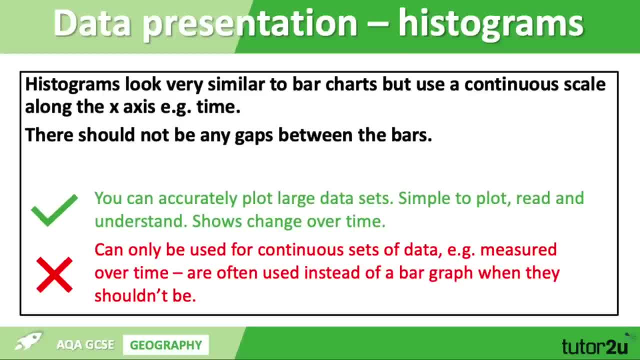 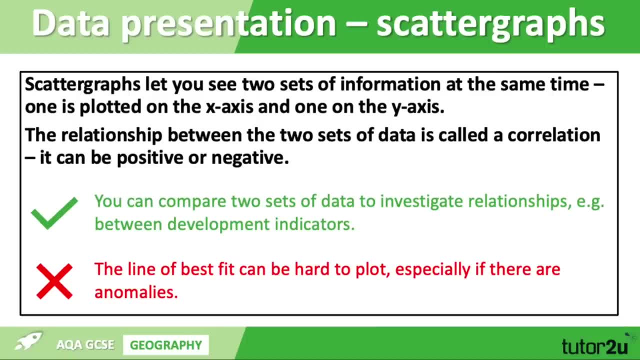 continuous sets of data, so the stuff that is measured over time, And quite often they are used instead of a bar graph, and they shouldn't be Right. let's have a look at scatter graphs Now. these let you see two sets of information at the 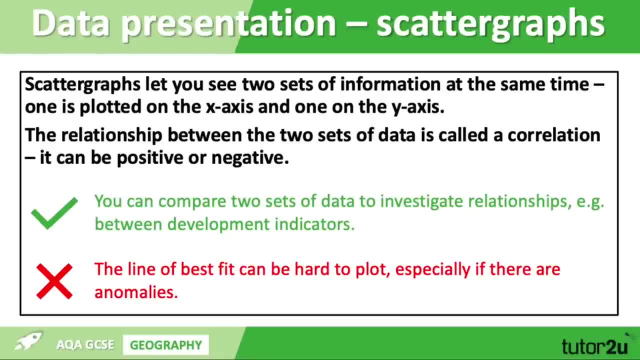 same time. One is plotted along the x-axis and one is plotted on the y-axis, And the whole point of a scatter graph is that it shows the relationship between two sets of data and what we refer to as a correlation, which can be positive or negative. So, in terms of positives, you can compare two. 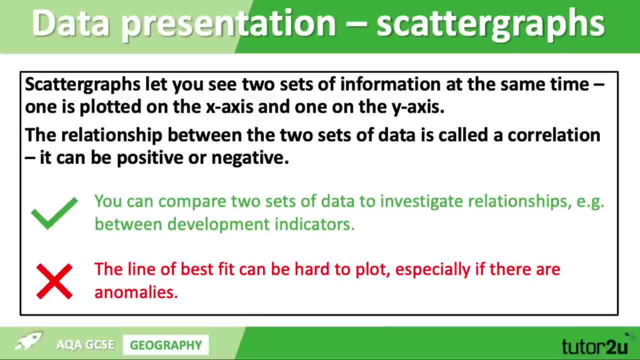 sets of data to investigate relationships such as between development indicators. but the line of best fit can be quite hard to plot, especially if there are anomalies. Now, with a scatter graph question, you could be asked to complete some data by plotting some crosses on. you could be. 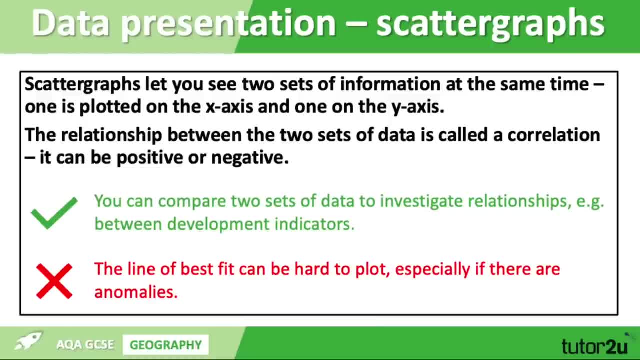 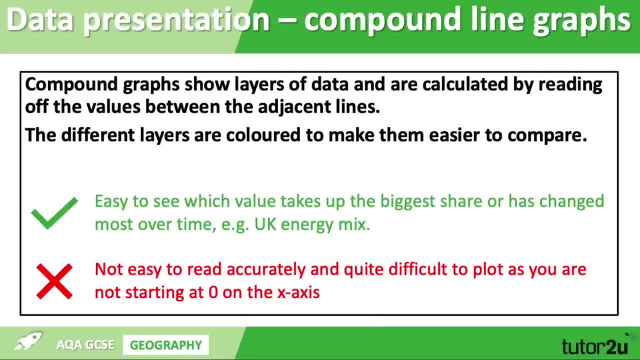 asked to plot a line of best fit, or you could just be asked to describe what the data is showing you Right? let's move on to compound line graphs. These are graphs that we see frequently in the exams. These show layers of data and are calculated by reading off the values between adjacent lines. 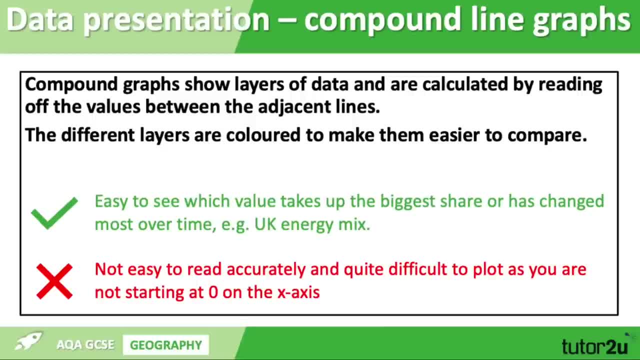 The different layers are coloured to make them easier to compare, so there will be a key that you need to read carefully Now. a benefit of them is it's easy to see which value takes up the biggest share or has changed mostly over time, So sometimes you'll have two of them next to each. 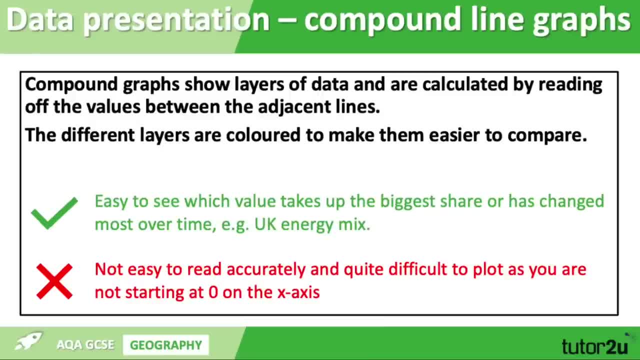 other and you're asked to show how something has changed. So, for example, it might be a graph showing the UK energy mix in 2010 compared to 1980. So you might be asked to think about how fossil fuel colour has changed compared to the nuclear colour, compared to the renewables colour. 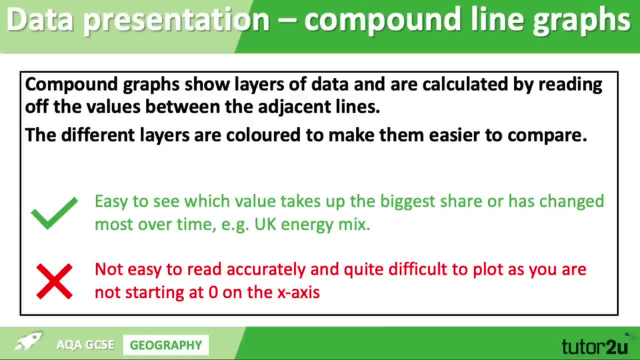 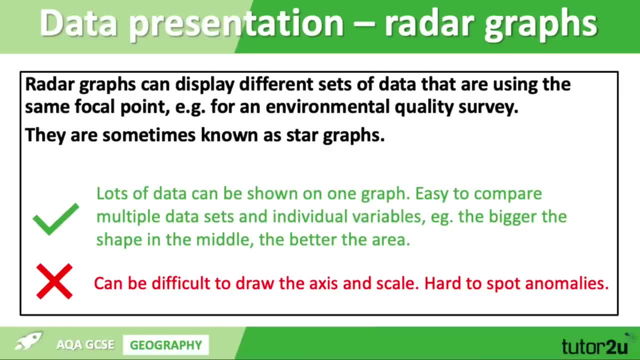 But they're not always that easy to read accurately and they're quite difficult to plot, as you're not starting at zero on the x-axis. Now, lots of you will be familiar with radar graphs. These are graphs that can display different sets of data that are using the same focal point. So you may 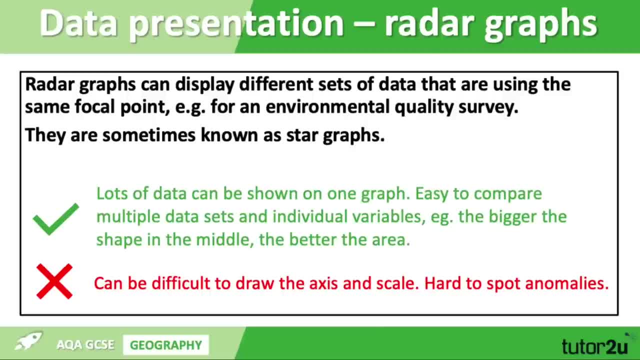 have drawn them for environmental quality surveys. They are sometimes known as star graphs because they look like a star when you're making them Now. they're useful because you can display lots of data on one graph, easy to compare multiple data sets and individual variables. because the 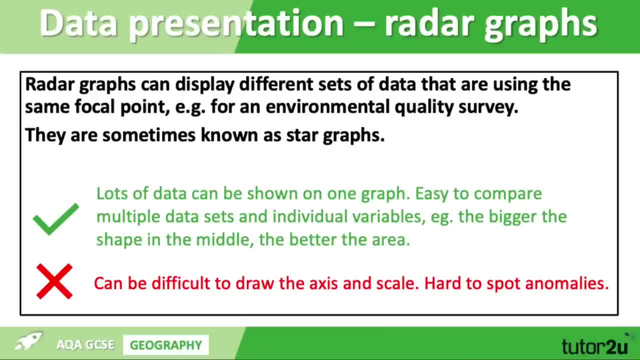 bigger the shape in the middle, the better the area, But they are quite difficult to draw in terms of the axis and the scale, and it's quite difficult to spot anomalies on them Right, our final data presentation technique that we're going to have to think about now is the use. 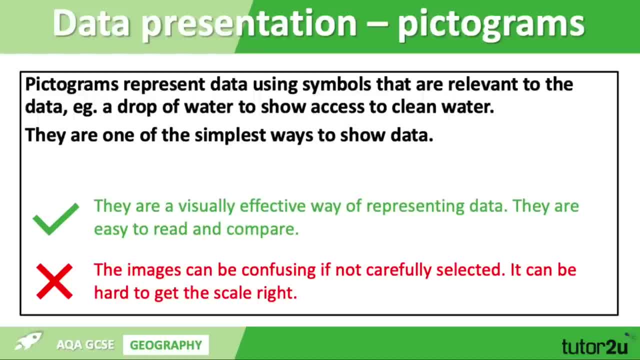 of pictograms. So pictograms represent data using symbols that are running in the middle of the graph and they are relevant to the data. For example, a drop of water might show access to clean water. They are a really simple way to show data and they are often used in the exam. One of 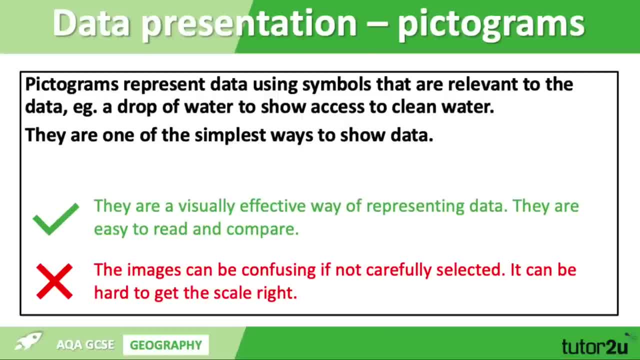 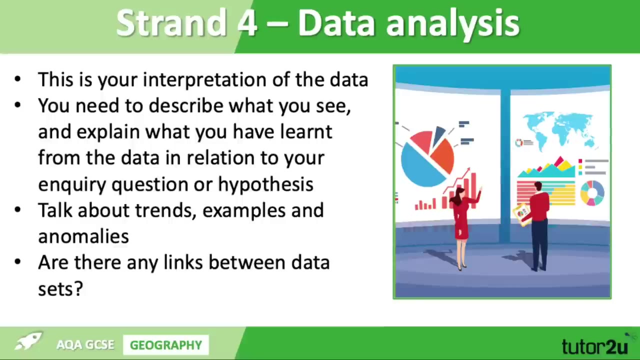 their biggest advantages are that they are really visually effective and they're really easy to read and compare. But the images can be confusing if they're not carefully selected and it is quite difficult to get the scale right. So let's look at strand four. Strand four is data analysis, which is describing, analysing and 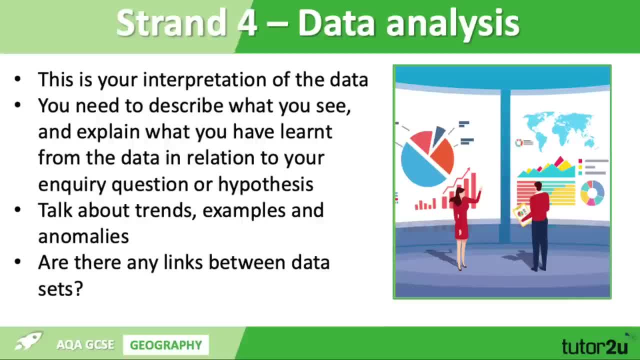 explaining fieldwork data. This is your interpretation of the data. You need to describe what you see and explain what you have learned from the data in relation to your inquiry question or hypothesis. It's about talking about trends, examples and anomalies and whether there are any links between 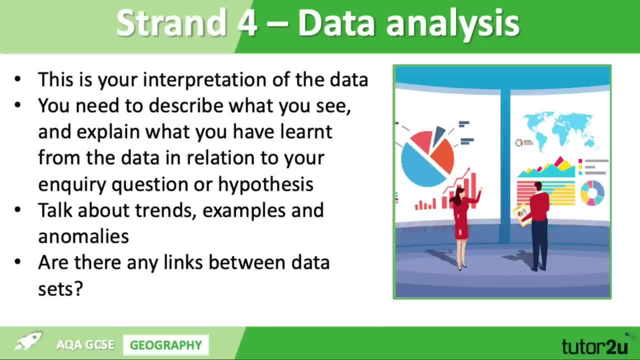 data sets. In the exam, you may be asked to describe, analyse and explain the results of fieldwork data. establish links between data sets and explain the results of fieldwork data. This is a very simple process. Use appropriate statistical techniques and identify anomalies in fieldwork data. An example exam: 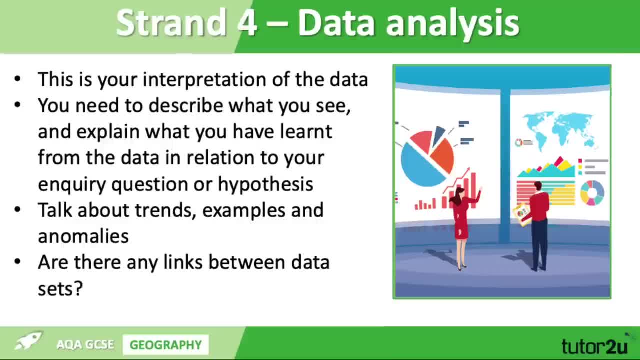 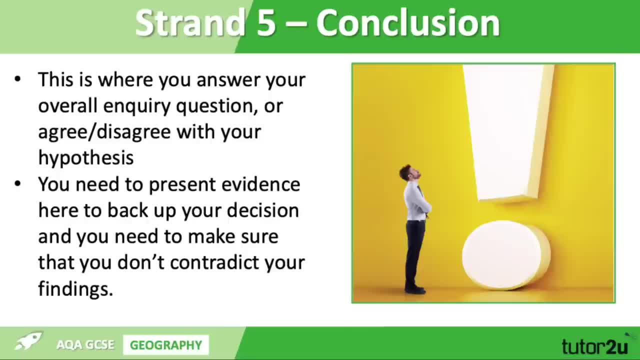 question here is assess the importance of establishing links between data sets. interpreting your physical geography fieldwork data. Three marks Right. let's move on to strands five and six, the conclusion and evaluation. These are often together in the final exam and they're usually the focus of the nine-mark question. 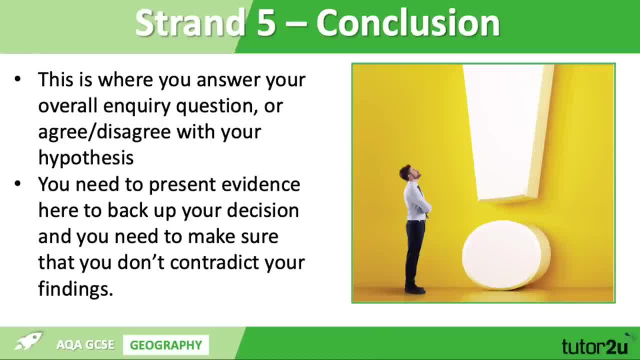 So what is the conclusion? Well, the conclusion is where you answer your overall inquiry question or agree or disagree with your hypothesis. You need to present evidence here to back up your decision and you need to make sure that you don't contradict your findings. 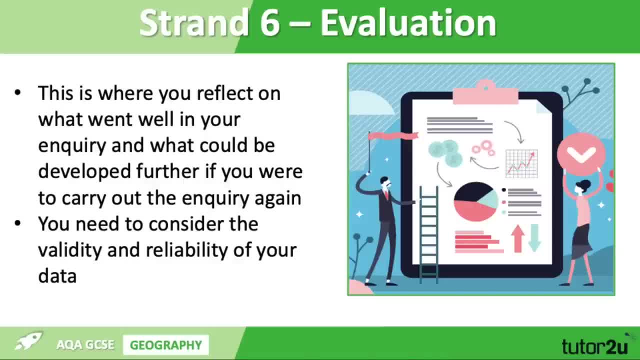 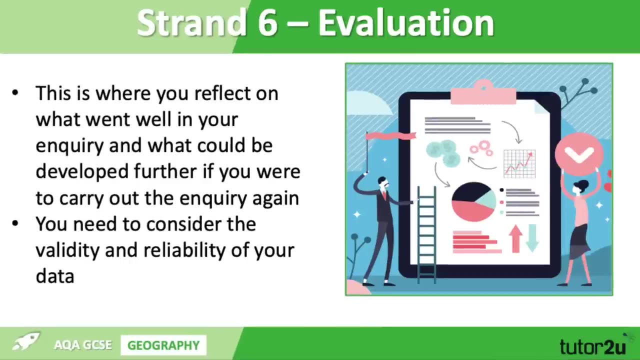 So how does the evaluation differ from the conclusion? The evaluation is where you reflect on what went well in your inquiry and what could be developed further if you were to carry out the inquiry again. You need to consider the validity and reliability of your data. In the exam, you will be expected to draw evidence. 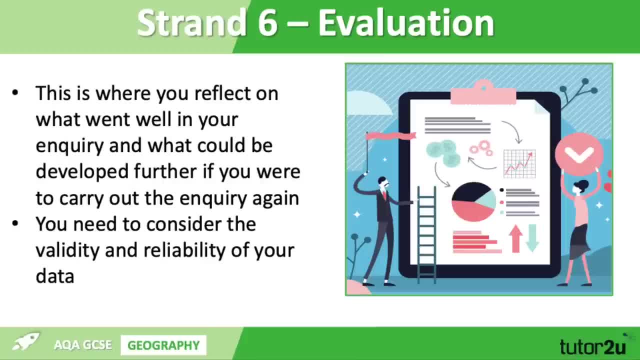 conclusions in relation to the original aims of your inquiries. You will also be expected to be able to identify problems with your data collection methods. limitations of data collected suggest other data that might be used and suggest the extent to which your conclusions are reliable.